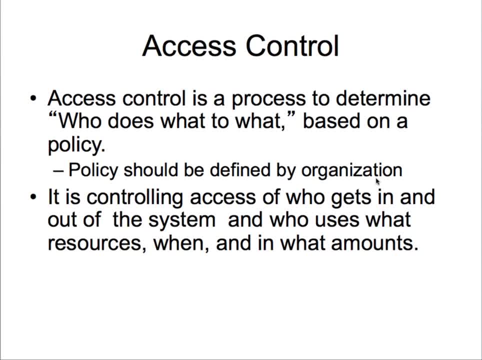 So essentially, access control is who gets in and out of a system and who uses it. It's what resources, when and in what amounts. If you think about it, that's a lot more complicated than what we discussed in the Linux administration course. 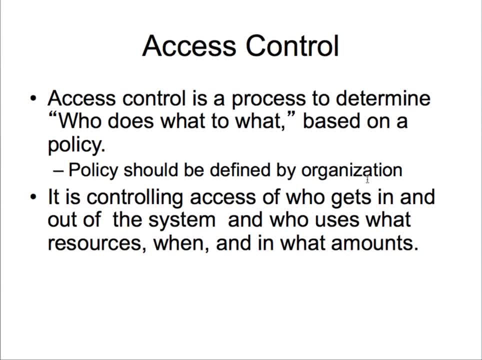 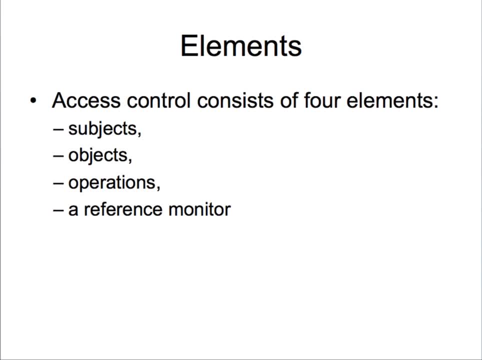 And it'll make a lot more sense when you see that access control is not just something that simple or doesn't necessarily need to be that simple. So elements of access control consist of the following four things: There are subjects, objects, operations and something called a reference monitor, which I didn't discuss previously. 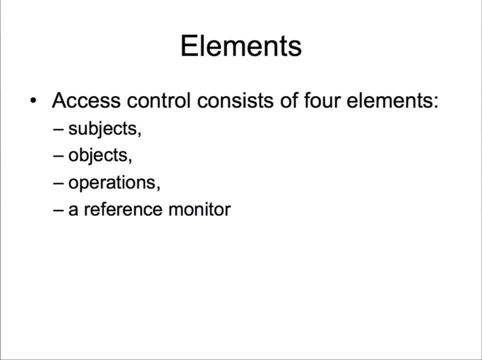 Now we already think about subjects. Subjects are going to be the users, as we discussed in the Linux administration. So what are objects? Well, objects pertain to something just as simple as files, but they could be other types of research sources, such as getting access to the printing server or getting access to a database. 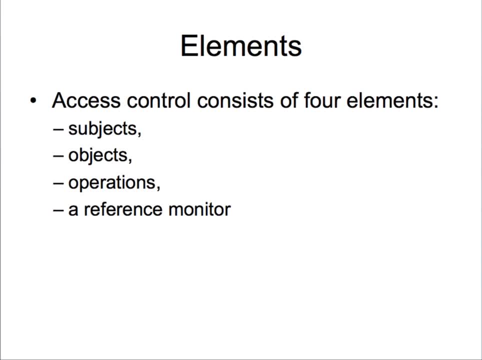 Operations indicate the ability of a subject to either access or not be able to access an object, Or even a subject accessing an object by a time or place or something of that nature. Then we have something called a reference monitor, and I will discuss that in a couple of slides in a little more explicit detail. 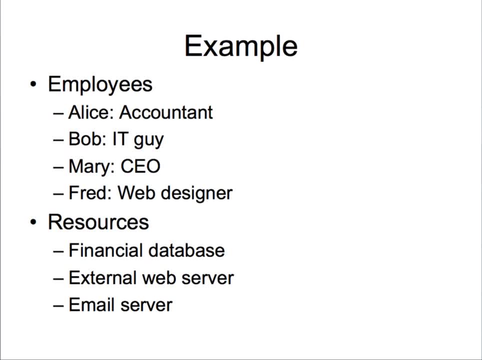 But just as an example, let's say we have a company, XYZ, and it has four employees: Alice is the accountant, Bob is the IT guy, Mary is the CEO and Fred is the web designer. Now, in this very simple example, there are various resources the company has, such as a financial database, an external web server and an email server. 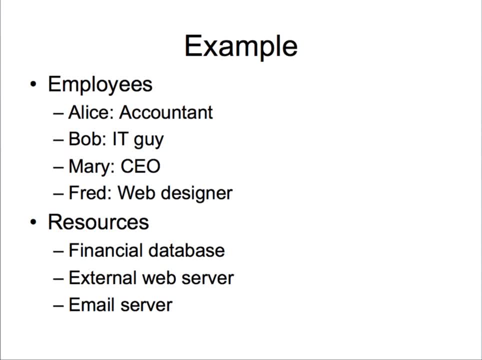 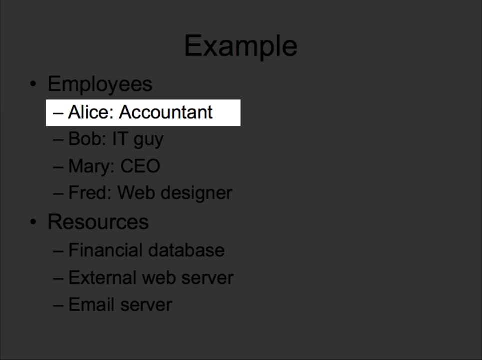 So if we think about controlling access to these resources, how would we go about determining whether a, let's say, Alice what she should have access to as an accountant? Well, if you look at the resources, maybe the financial database, Yeah, that kind of makes sense. 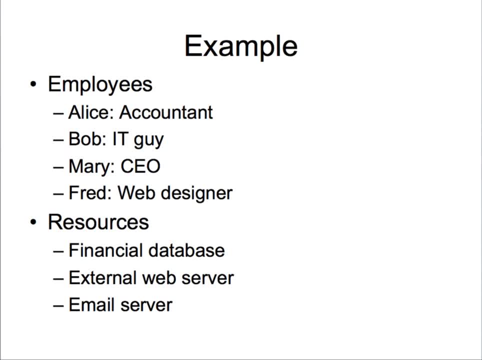 What about the external web server? Would she need access to that? Well, probably not, But regardless, her ability to access any of these resources should be defined explicitly in the access control policy as created by the company. How about Bob the IT guy? 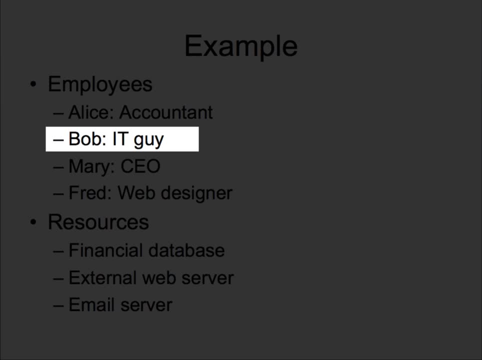 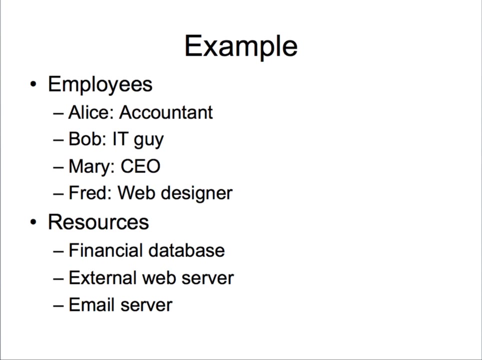 Does Bob need to get into the financial database? Well, probably not, But certainly you might give him access to the external web server So that he has at least some control over that. Who else on that list of employees might we want to be able to access the external web server? 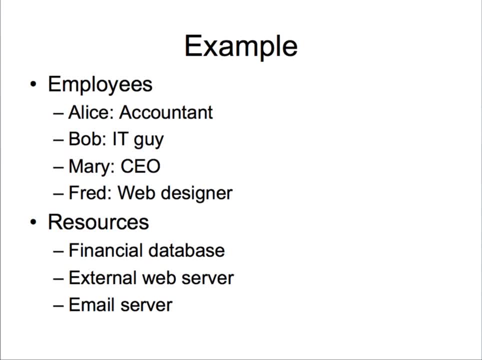 Well, certainly, Fred. Let's look at Mary the CEO. What should Mary be allowed to access? Financial database, Maybe External web server? Well, we might. It depends upon her level of sophistication and her need to be able to get into the external web server to make changes. 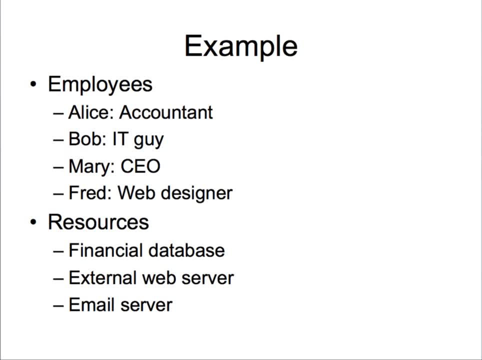 And, yeah sure, maybe everybody on the email server giving them, as we'll see later on, various levels of access to the email server. All levels of access aren't the same, as we'll see later on, But that's essentially what access control does, is it allows certain subjects to access certain objects in various levels of detail. 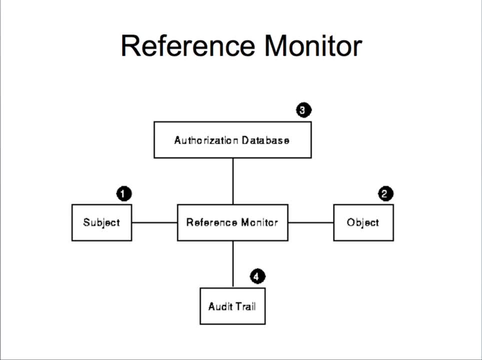 Now getting back to the reference monitor. what is a reference monitor? We talked about subjects and objects, For example, notice number four down there. We also have an audit trail, which is a good idea. It's something that we'll learn and you'll actually see later on when you'll see that when someone- a subject- is accessing an object, 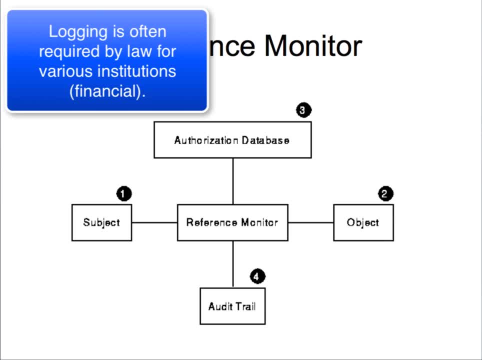 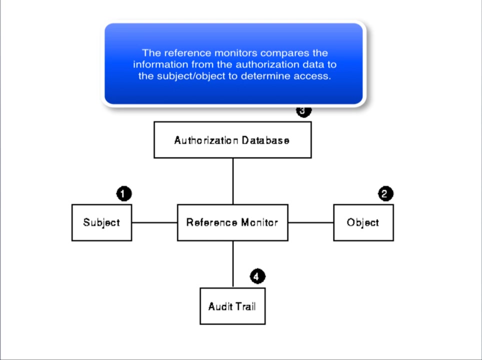 it's good to have a trail, an audit trail or a logging system that indicates whether that person was able to access the object. The reference monitor really ties in everything. It looks good. It contains those operations and rules, as we'll see later- that determines whether the subject is able to access the object and how they're able to do it. 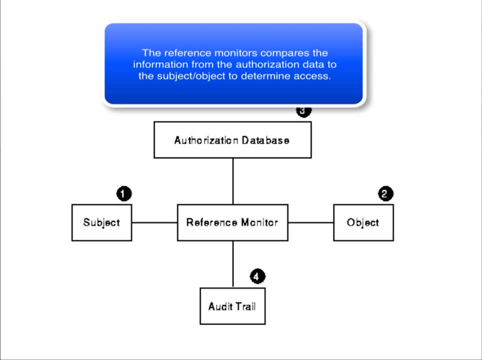 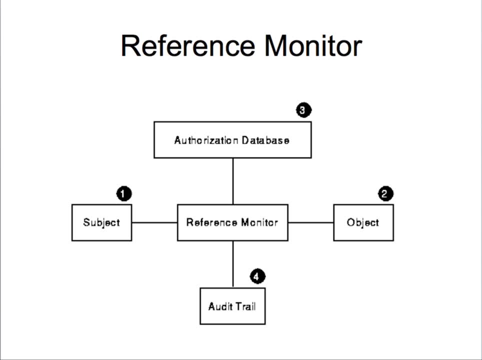 For example, when we looked at the Linux administration course, there were really only three sets of operations that a subject could perform on an object, And specifically we were looking at files. And what were those? Well, we had read, We had write. 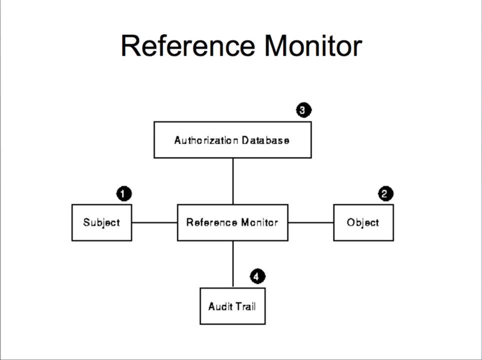 And we had execute Right And we saw that sometimes a certain subject was able to read, write and execute on a file And for other files they were only able to, for example, read that file, but they weren't able to write or execute that file. 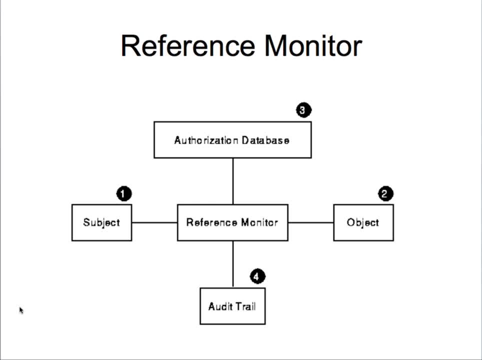 So all of that is determined by the authorization database, which indicates what the- let's say- I'm just using the term- in general- rules that allow a subject to interact With an object, And that reference monitor is the thing that actually applies that to the situation. 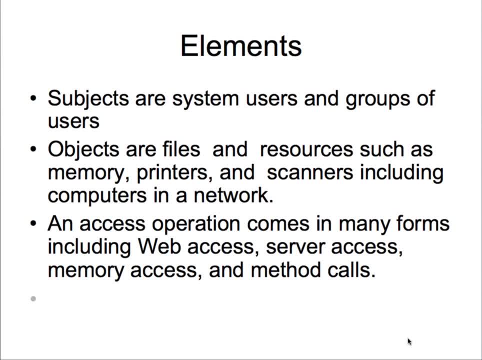 So just to be clear, here, the subjects are the system, users and groups of users. Recall from the Linux administration course is: you could put users in various groups, and that's how we were able to allow a number of users to be in a group. 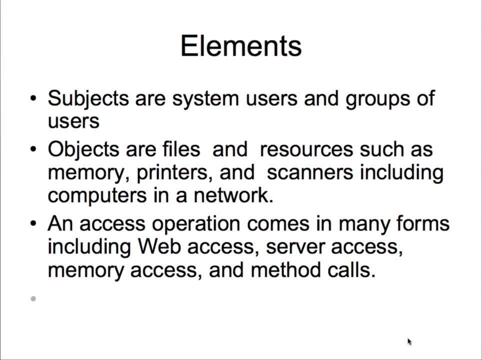 And then that group was able to access an object and perform operations on it. The objects are most typically, But they could be other resources such as memory printing and scanning, and even including other computers on a network. And an access operation again comes in many forms, including web access, server access, memory access and even method calls. 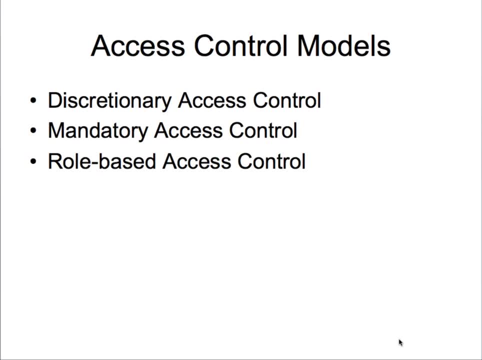 So let's look at the three access control models. We have discretionary, mandatory and role-based access control. Now, most of you are Most familiar, if you're working with Linux, Windows and the Macintosh, with the discretionary access control. 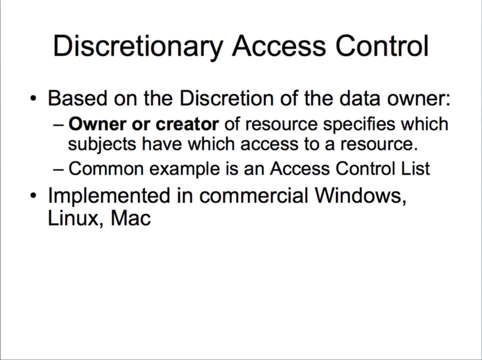 So discretionary access control is based on the discretion of the data owner, And that's what we saw in Linux- is that when we created a file, we were the owner, And so the owner or the creator of that file specifies which subjects have access to that resource. 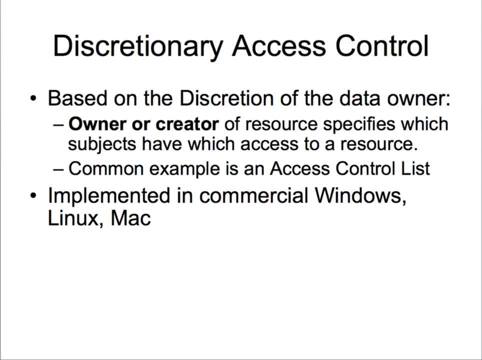 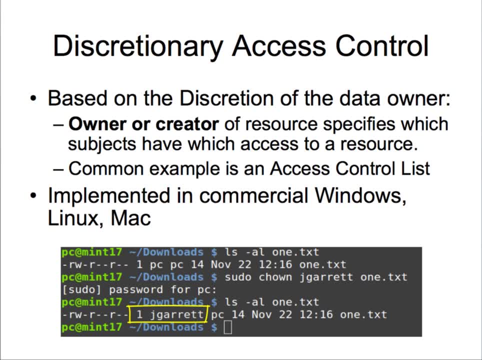 If you recall, when we were creating files, we were changing permissions on the file. We could even change Ownership of the file, And so that's the most simple level of access control, And an example of that is an access control list, which we'll talk about in a lot more detail a little later on. 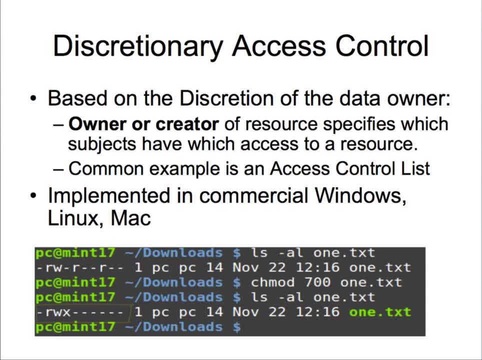 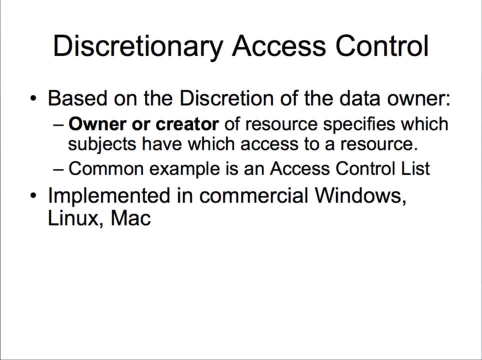 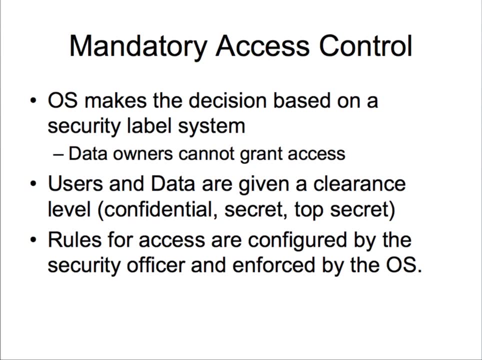 But suffice to say that Windows, Linux and the Mac and pretty much any Unix- with one stipulation, as we'll see later- implements discretionary access control, A more complicated form of access control. It's mandatory access control And that's where the operating system makes the decision as to whether a subject accesses an object, based on a security label system. 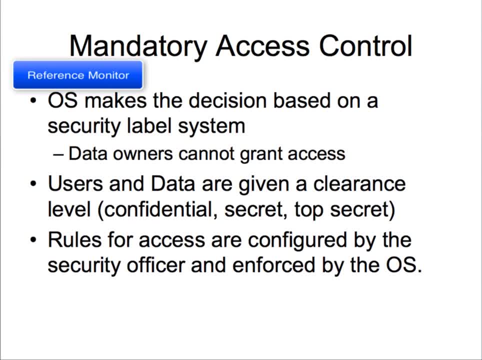 So it's the operating system, rather than the data owners or creators, that allow or disallow granting access to the object, And the best example of this is what we see in the military is where users and data are labeled According to a clearance level, for example, the confidential secret and top secret which I'm sure you've all, or at least a little bit, familiar with. 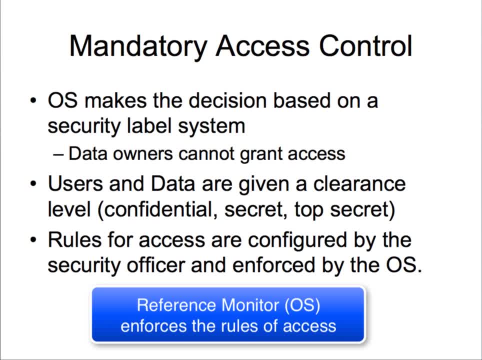 And then we have rules for access, which are configured by the security officer and then enforced by the operating system. And when I'm talking about the operating system, I'm talking about that, not only the authorization database that indicates who has access to what. 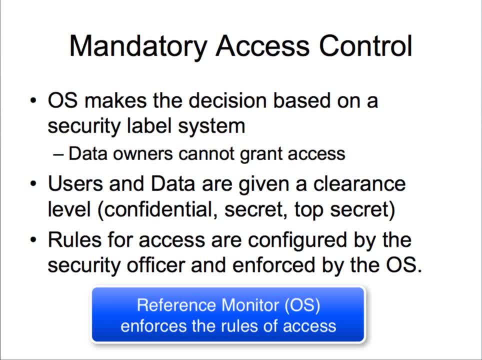 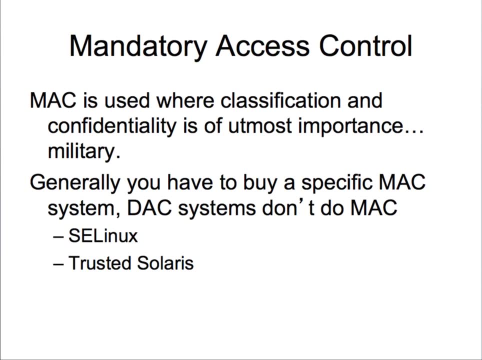 but also that reference monitor that looks at the authorization database as well as the Classification levels of the subjects and the objects, determine whether access can be granted. Macs are used for classification, and confidentiality is of the utmost importance, which the primary example would be the military. 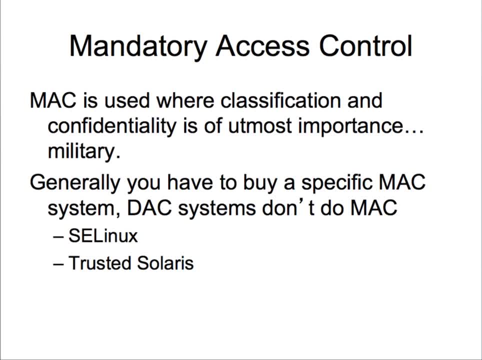 And generally you don't, You don't see mandatory access controls. when you buy a commercial, When you go out and you buy a Windows 10 computer or the latest Macintosh, is that you have to specifically buy or at least implement mandatory access control. 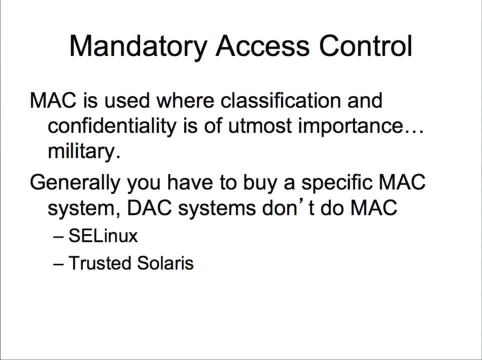 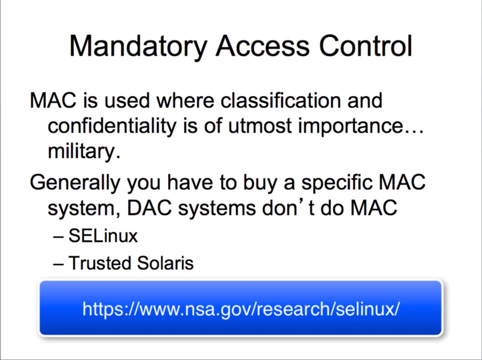 for example, with trusted Solaris or something called a secure enhanced Linux, which was created by the National Security Agency, And that's actually something that you can download from a website and implement on your Linux system. I would suggest that you You do a lot of research on that and read up a lot about it before you do that, because it's a good way to lock yourself out. 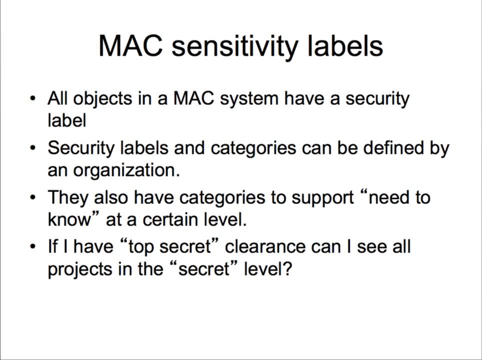 So all mandatory access control systems have a security label And those labels, as we saw before, at least in the military, are confidential, secret and top secret, And those security labels in the categories are typically defined by an organization, In this case the military. 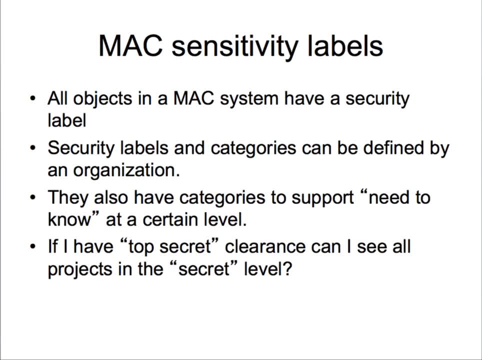 And there's also one more category which goes above and beyond the Mac label, And that is whether you have a need to know at a certain label, And we'll talk about that in a second. The question is if we're talking about the security labels or security designations of confidential, secret and top secret. 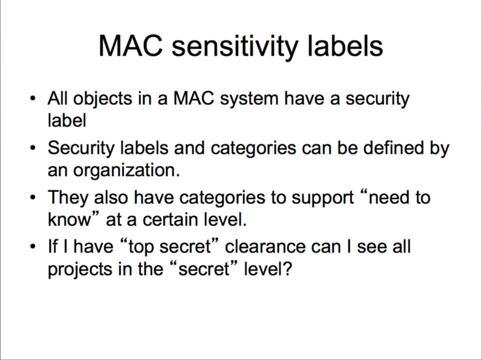 if I have a top security clearance, can I see all of the projects in the secret level? And typically the answer is No. Not only must your security clearance be equivalent to that as designated to the object, but also you have to have a reason to access that information. 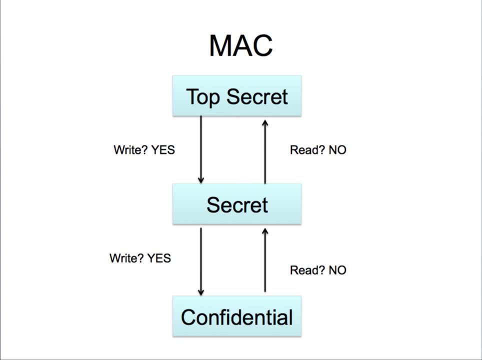 You have to have a need to know. As we see here on the screen, we have the three security clearance levels, as well as the sensitivity designation of confidential, secret and top secret, And so Let's say, as an example, we have a let's say for this example. 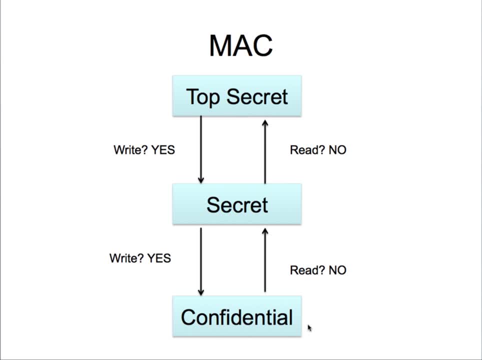 is that you have a confidential security clearance and you need to look at a memo that has been designated as confidential. As long as you have a need to know, you're able to view that memo. As another example, let's say that an object has been. 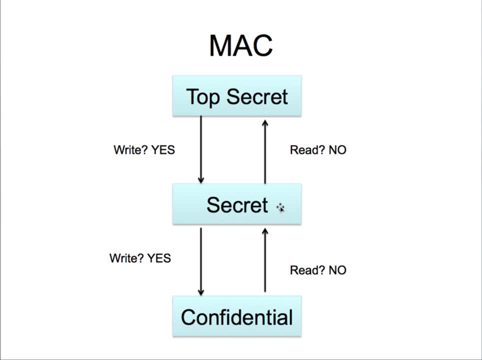 been deemed at this with a security label of secret and you only have a confidential clearance. Can you read the secret level memo? The answer is no. Can you read the top secret level? No. So in other words, notice that you can't read up. 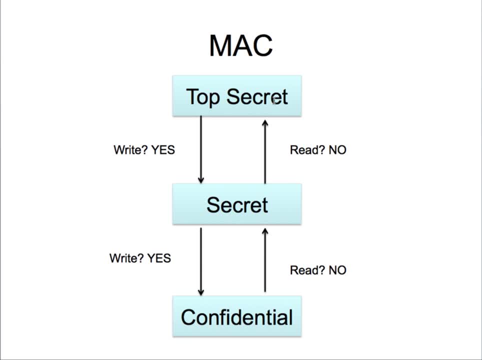 Someone who has a secret level clearance cannot read a top secret memo, And I change this to make this clear, Because actually I was trying to combine two separate concepts. so what I did was I paused the video and I changed what you saw on the screen. 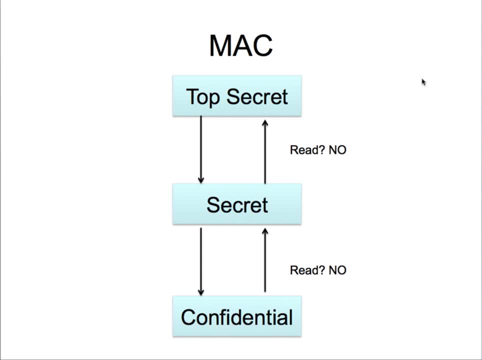 And I'll explain that on the next screen. So this: so we see that we can't read up So confidential, can't read anything secret, Secret. can't read anything top secret, even though they might have a need to know for some particular reason. 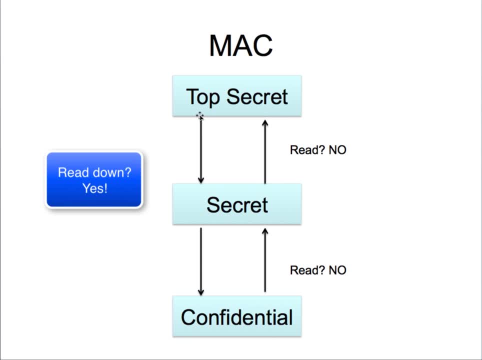 Does. how does it work the other way, though? What this is indicating- that the arrows on here on the left- is that somebody who has a top secret clearance can not only really read a top secret memo. they can also read a secret memo and also a confidential memo, as long as they have a need to know. 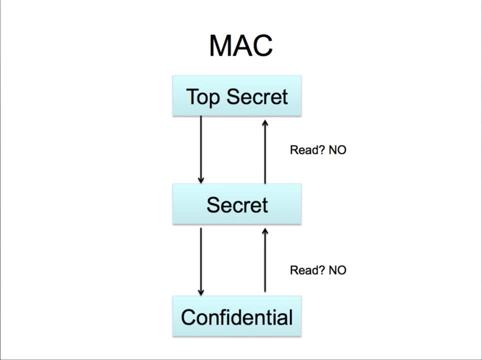 Now think about producers of objects. That is now someone with a confidential, a confidential security clearance. creates an object somehow- and it can- and it happens all the time- that is later deemed secret. at the time they don't know that it's going to be classified secret, but they create one that's secret. 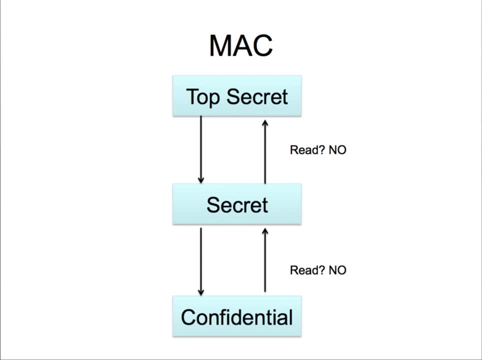 And I've known this from a personal circumstances, not me, but with other people. So somebody who has a confidential security clearance, can they actually create a document that is later deemed secret? Yes, they can. So essentially what this is saying is, as that you can write up. 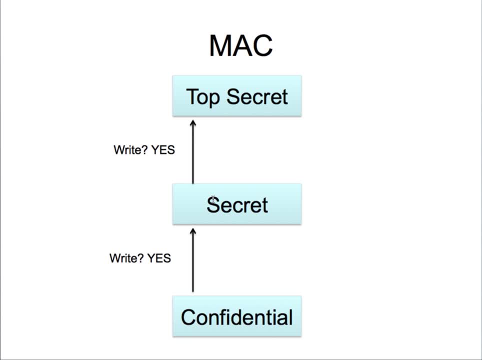 so you can create one that's secret. or if you're secret, you can create one that's top secret. Or even if you're confidential security clearance, you can write one that's top secret, But guess what? You would no longer be able to read it. 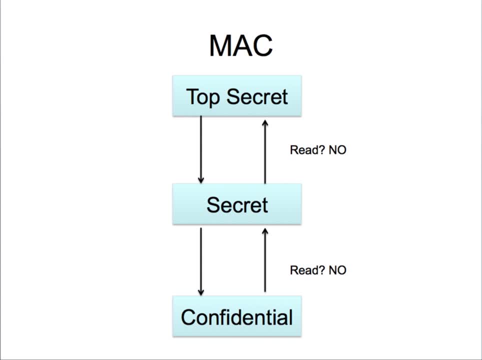 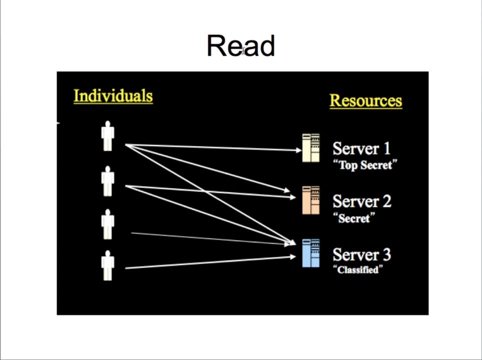 I'm afraid that's a fact. I know that sounds weird, but that's absolutely true. And this is just another graphical depiction of what you see here, And this is when we're talking about reading, And this also is predicated on the background that these people, these little icons here 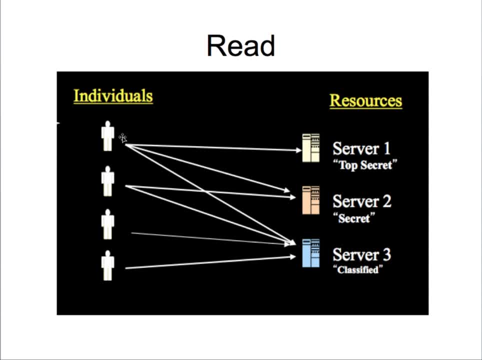 are individuals who have, for example here, a top secret clearance- This guy right here, this lady- they can read this resource And actually it's kind of weird the way this is written. This almost looks like it's a right. 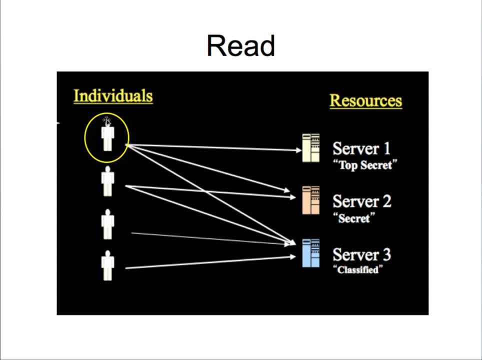 But what they're talking about is accessing the server one which is top secret. So this person is top secret, so they can access the top secret server. They can also access the secret level server two, as well as the classified or confidential server. 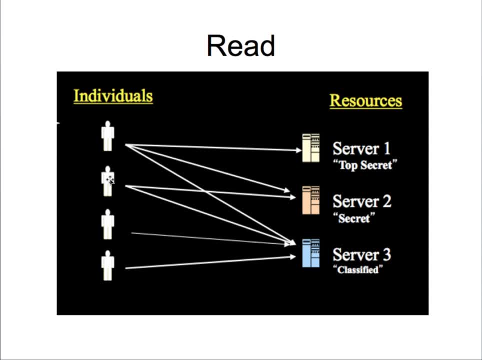 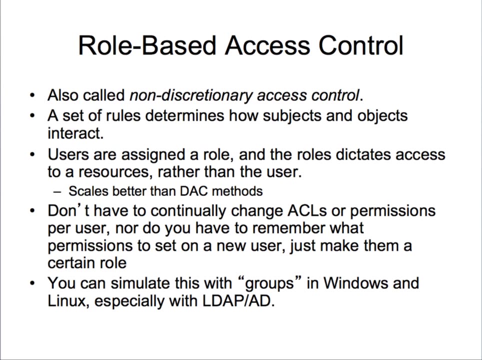 And notice as you move down this hierarchy here is that the secret clearance individual can access the secret and the classified, But notice that they can't read up. They're not able to read up And a third type of access control is called role-based access control. 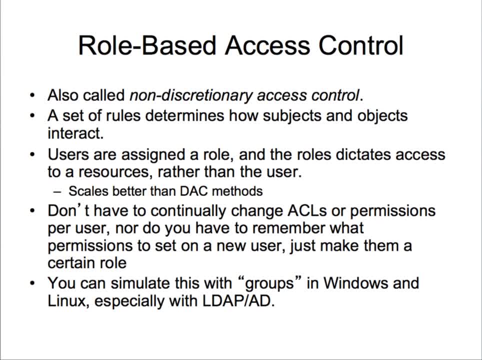 And it's also often called the non-discretionary access control, And essentially it's creating a set of rules to determine how subjects and objects interact, And so users are assigned a role, and the roles dictate access to a resource rather than a user. 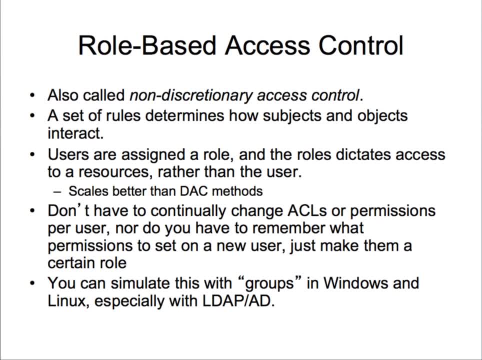 And it scales much better than discretionary access control, because you don't have to continually change the access control list- which again I'll talk about shortly- or the permissions per user, nor do you have to remember what permissions are set on a new user. 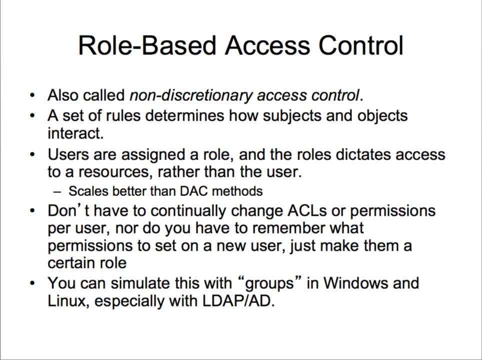 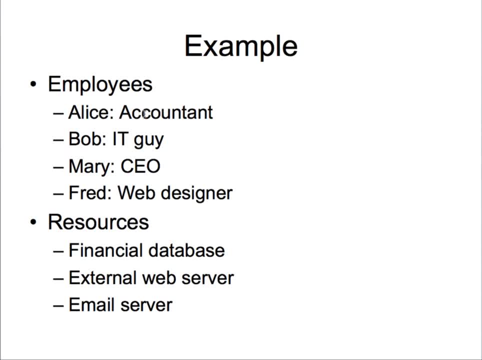 just make them a certain role, For example up here. let's go back to this example right here. And so these are the roles here. Notice, there's an account role, there's an IT role, there's a CEO role and a web designer role, And previously we identified: 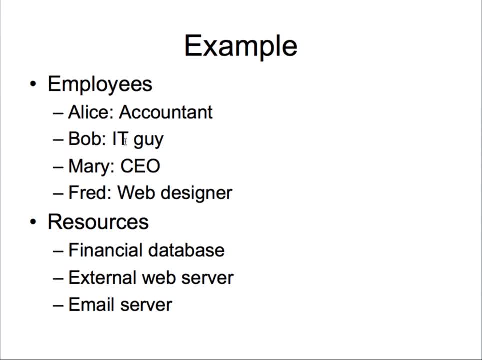 these users' access to these resources or objects down here. So what if, later on, Alice, who shouldn't be able to access the external web server or email server, moves to IT? How would we change this? Well, we don't want to go in and start changing. 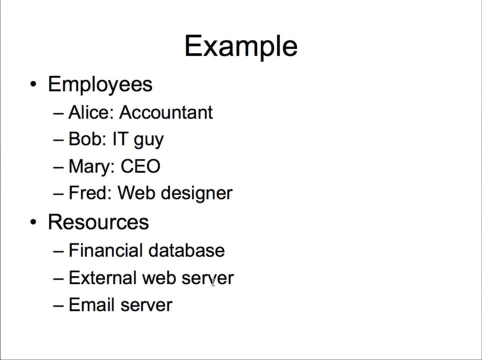 the permissions on the financial database or the external web server or the email server. It's better to set up predefined roles that suggest that there's an accountant role and all accountants who are a member of this role have access to the financial database. 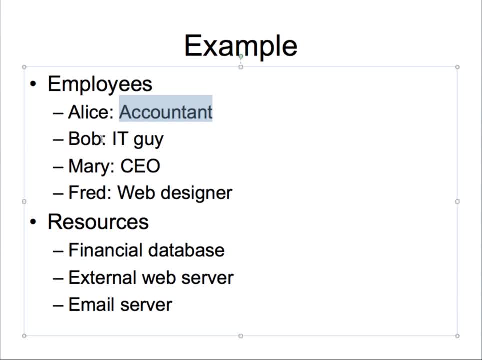 database and the database only. But later on, if Alice moves on up to be- and I say an IT guy, I use that in a general sense- and we hire somebody called Ted to become an accountant, well we don't have to go back and change any of the permissions on. 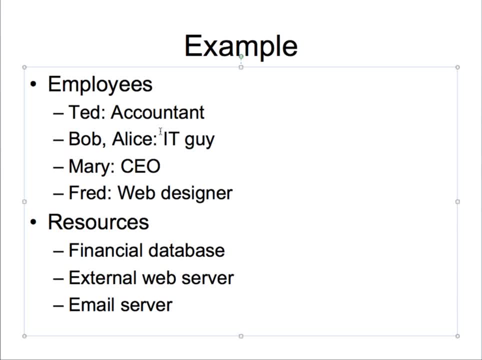 any of these objects. All we have to do is to put Ted in the accountant role, and Alice now no longer has access to the financial database, but she does have access to the external web server and maybe even parts of the email server, and now Ted has access to. 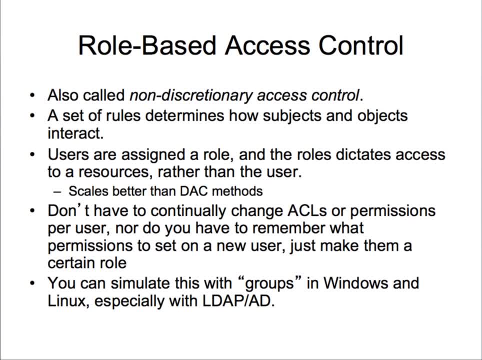 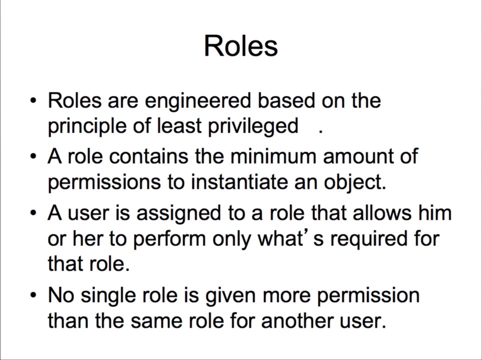 the financial database. You see how that works much more cleanly and scales better than the discretionary access control. You can simulate this with groups and Windows and Linux, especially with LDAP and Active Directory, And roles are engineered based on the principle of something called least. 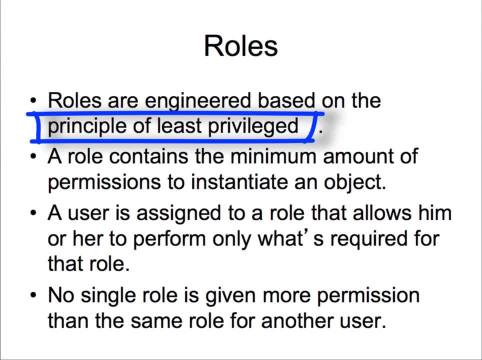 privilege, which you should have read about in another class and in your book, And least privilege just means that the user should only have access to stuff that they need to do their job And that actually, if you think about it, speaks to the need to know idea as well. For 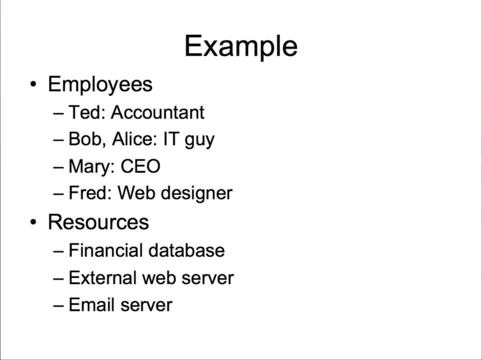 example here. what does Ted need access to? Well, the least privilege should be: in order to do his job, he needs to be able to access the financial database. He doesn't need, for his job, to be able to access the external web server. If he did, we could go back and 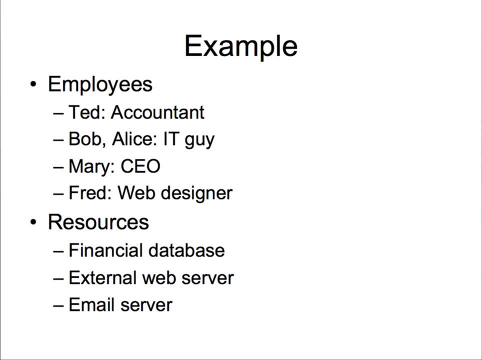 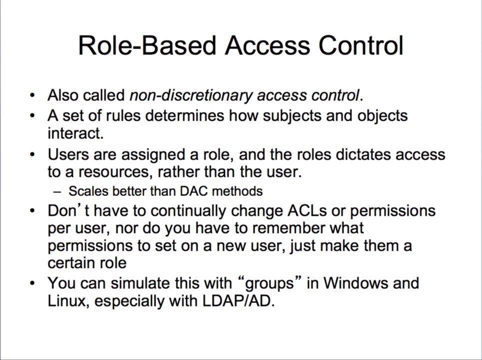 change the role of accountant so that now the accountant could access both the financial database and the external web server. That's what they need to do, And so least privilege is a core concept in information security, and it's something that shouldn't be taken lightly. 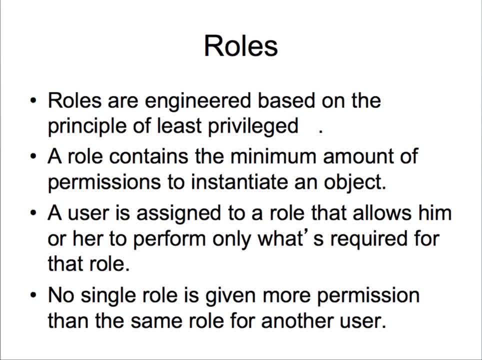 Let's go back here. So the role contains the minimum amount of permissions to instantiate an object, to create an object or to manipulate an object. A user is assigned to a role that allows him or her to perform only what's required for that role and for nothing else. 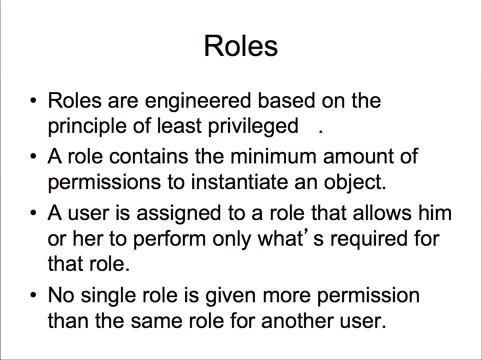 And no single role is given more permission than the same role for another user, And that's the whole idea. An accountant- anyone who is set up in the accountant role- should have the same permissions as every other accountant. If you had different levels of account, let's say an account one person who deals with the 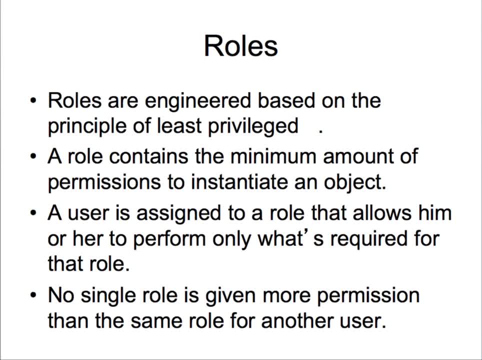 various aspects of a company and then you have an accountant two that deals with other aspects. Those would be two different things. They would have distinct roles and one may be given more permission than the other, but everyone within the accountant one role would have the same exact permissions and everybody. 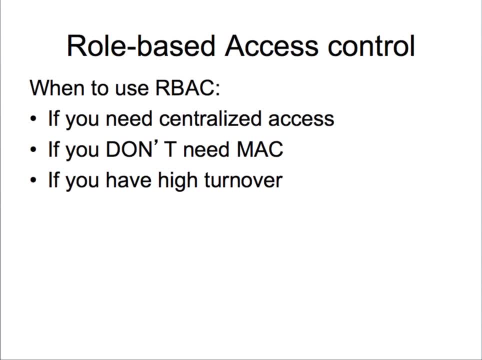 in the account. two role would also have the same exact permissions. So when would you use a role-based access control? One if you don't need centralized access, If you don't need something as complex as mandatory access control And, of course, if you have high turnover, if you're constantly churning and changing jobs. 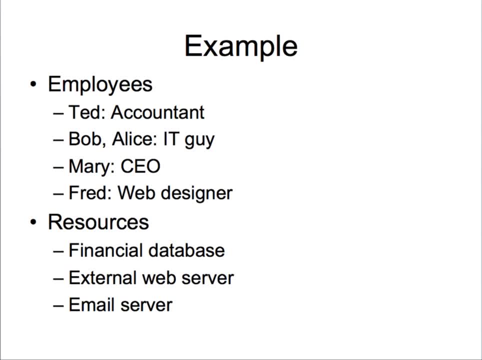 in here. Let me go back here. If every six months, these people are moving around or they're being fired and you're adding new people, rather than looking at discretionary access model, where you're constantly changing permissions here on the users and on the objects, all you're having to do is put people in the 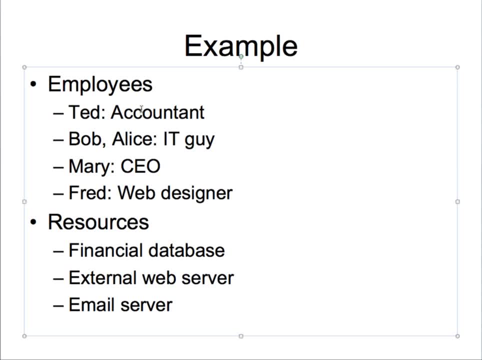 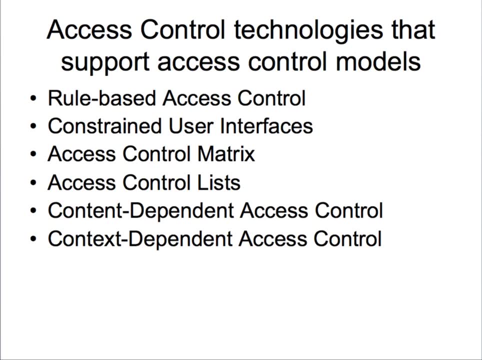 different roles. You're either putting them in the account role or you're taking them out of the account role. Okay, now let's talk about access control technologies that support what we've discussed before in terms of access control models, Rule-based constrained user interfaces, access control matrices, access control lists, content. 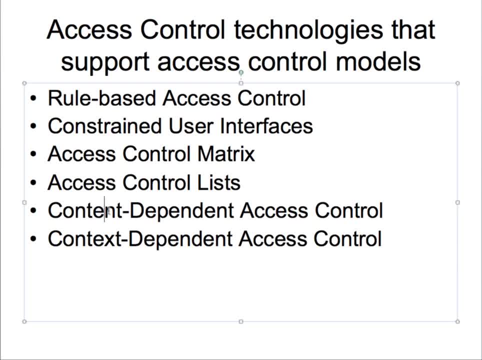 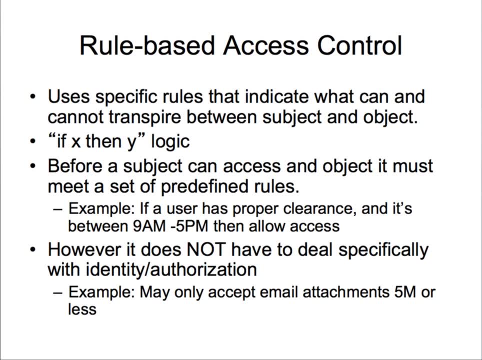 dependent access control and context. Notice that there's an N here and there's an X: Content versus context. Okay, So rule-based access control uses specific rules that indicate what can and cannot transpire between a subject and object. That is simply the logic that you've seen in your math classes or your computer science. 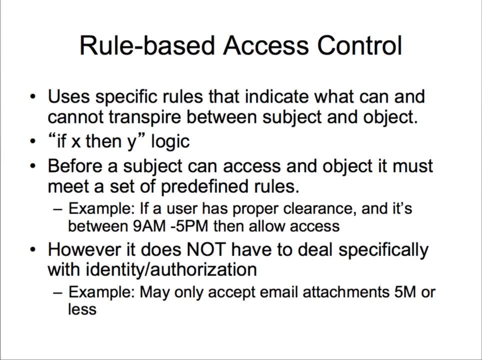 classes. If X, then Y logic. So before a subject can access an object it must meet a set of predefined rules. For example, If a user has a proper security clearance and it's between 9 am and 5 pm, then allow. 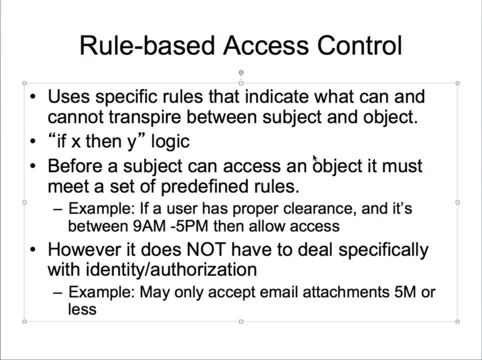 access. Now notice how, now our rules are becoming more complicated. Not only must a person have, for example here, the proper clearance, they have to have a need to know, and now we're setting time limits, So that makes a lot of sense. 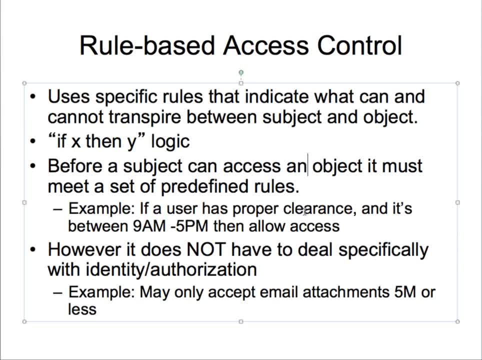 For example, if no one is allowed external access from, for example, an external IP address to a certain database And they're only supposed to be working during the day, Then instantiating this rule here: 9 am to 5 pm, if that's their standard working. 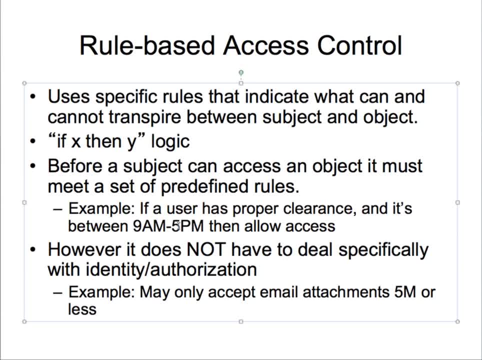 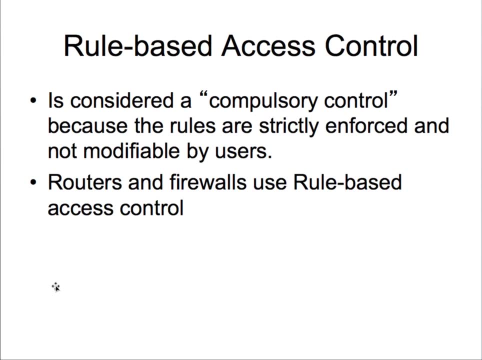 day And they're coming from the right IP address in the company, then they would be allowed access. Otherwise they would be denied. However, rule-based access control doesn't necessarily deal specifically with identity and author, So rule-based access control is considered a compulsory control. 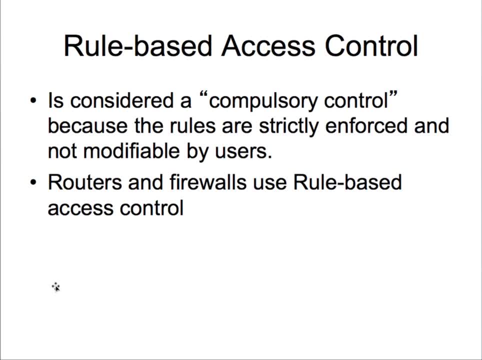 Okay, So the rules are strictly enforced and not modifiable by the users. So if you think about routers and firewalls- and firewalls we will look at in a little bit- you'll see how we will create rules that set up restrictions to certain objects. 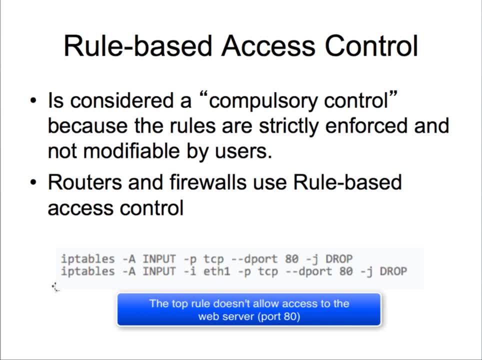 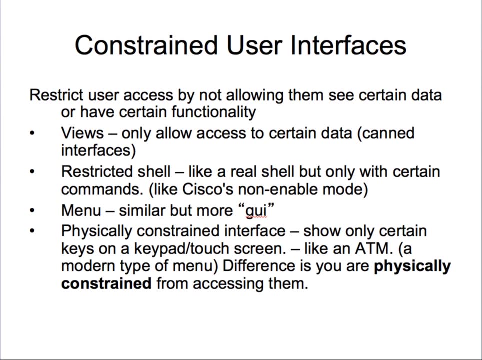 For example, a telnet server or an FTP server. What is the source address? What is the source port? We define rules based on that information to allow or deny access. And here's something that, if you think about access control technologies, we see all the 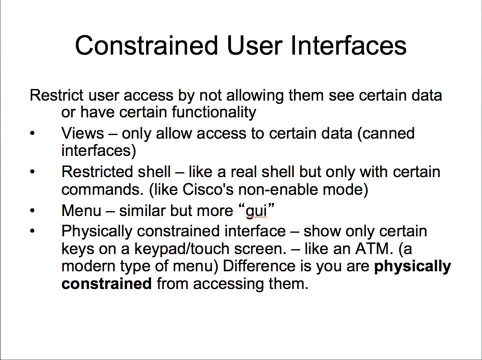 time, For example, a constrained user interface. We can restrict user access by not allowing them to see certain data or have certain functionality on the computer, And this can come in many examples. For example, views only allow access to certain data, that is, canned, interfaces that only. 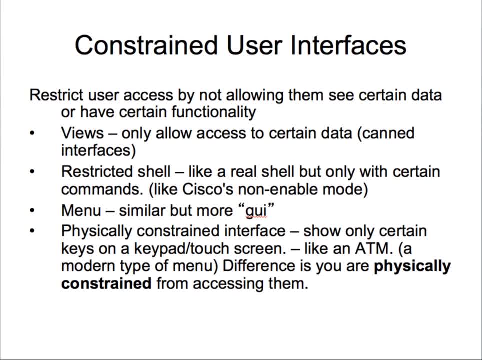 show a user specific information and they hide everything else to which they should not be allowed access. We can also give them something called a restricted shell. So a shell is the terminal, as we used in Linux administration and in this course as well. So it's like a real shell, but only with certain commands that are enabled, like Cisco's. 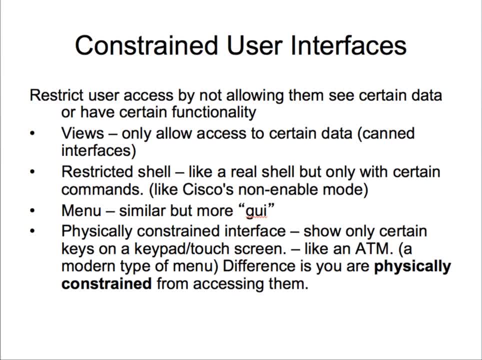 One that's highly restrictive is the menuing system, and we'll see it on a separate page here And so now we're talking about a graphical user interface where we can give access to certain objects at varying levels of detail based upon that person's status in the organization. 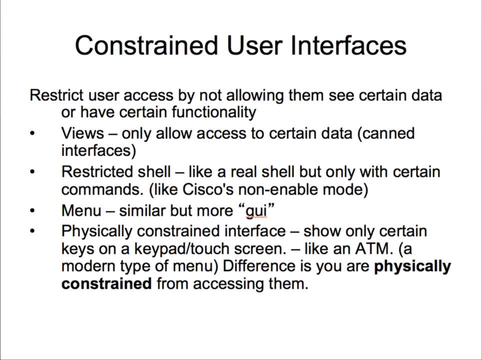 and that's all limited by the menuing system, And we can also have physically constrained interfaces that show only certain keys on a keypad or a touch screen like an ATM. So the difference is here is that users are being physically constrained from accessing data as either viewing or manipulating the object. 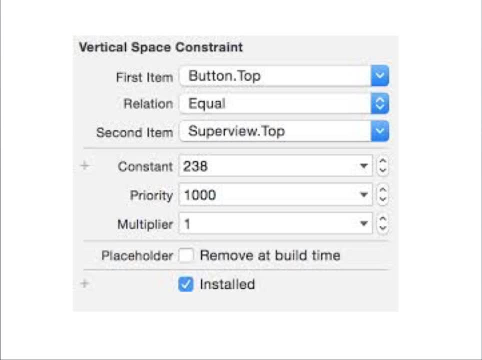 So if you see something like this, what is the user allowed to do on here? Well, it's constrained by the user interface, as they have drop-down menus where they're allowed to only select, for example, on these top three lines. right here they are allowed. 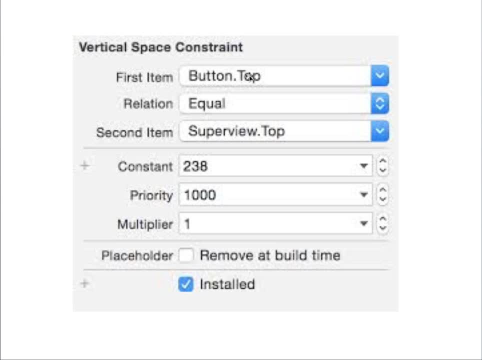 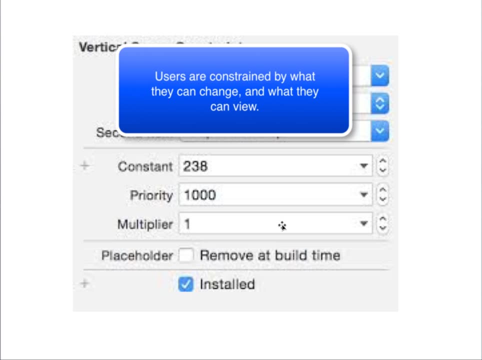 to select certain items. They're not allowed to select anything else. and the same thing down here. Now we're talking about numerical input, And that's what we're talking about. And that's what we're talking about, And that's constrained as well, and they can either click here or here, but this is all. 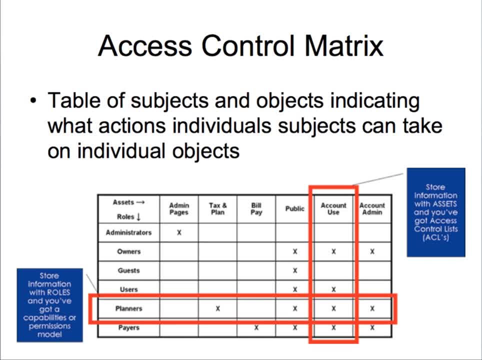 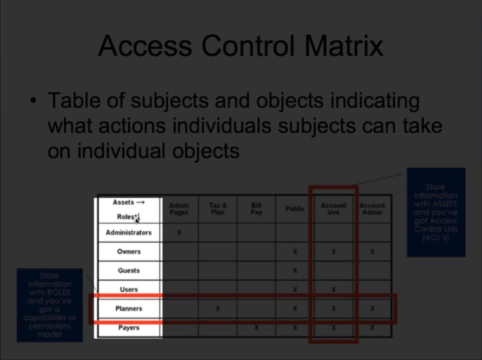 constrained by the user interface. So this is an access control matrix, which is a table of subjects and objects indicating what actions individual subjects can take on individual objects. So, going down in the columns, in the first column over here you see the roles: administrators. 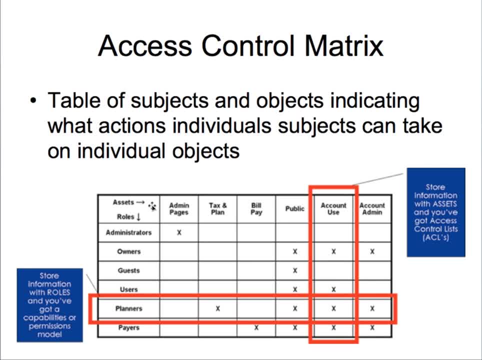 owners, guests, users, planners and payers. On the top, going across this row, we have administrative pages: tax and plan bill pay, public account use and account administration. So if we divide this up by rows and columns, we get either a capability table or an access. 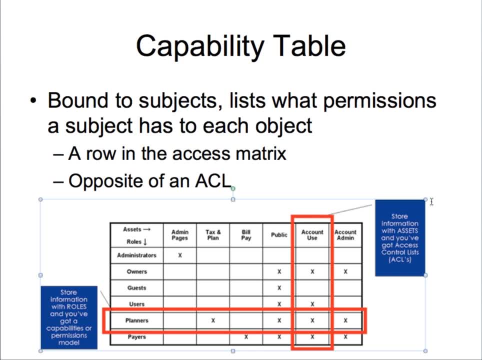 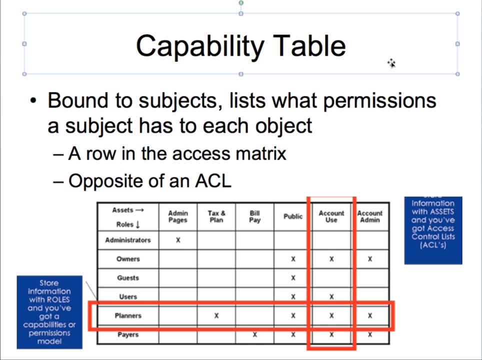 control list. So let me make this a little bigger, if I can. So a capability table is bound to the subjects. So now we're talking about this first row over here- administrators, owners, guests and so on- And it lists what permissions a subject has to each object. 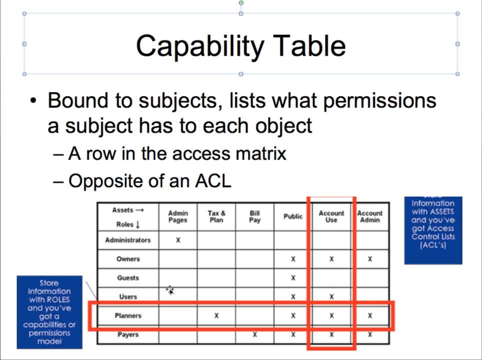 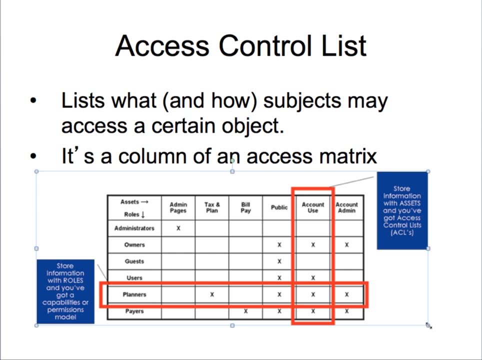 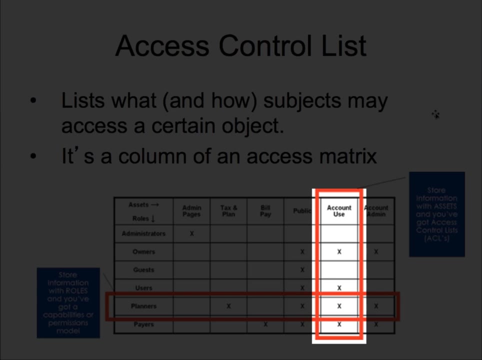 So it's a row and it's the opposite of an access control list that we'll see shortly. So planners have permissions to access tax plan, public account use and account administration. An access control list now looks in the columns. Now we're talking about lists, access control lists. 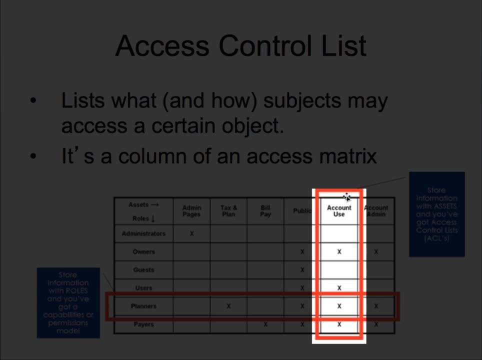 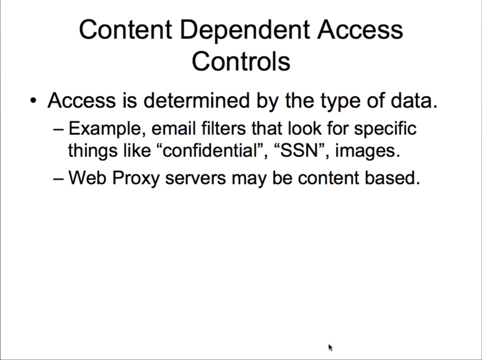 What and how. So the list of the objects may access a certain object. So now we're talking about columns. So the account use indicates who has access to this resource, which would be owners, users, planners and payers. Another type of access control technology is the content dependent access control, which